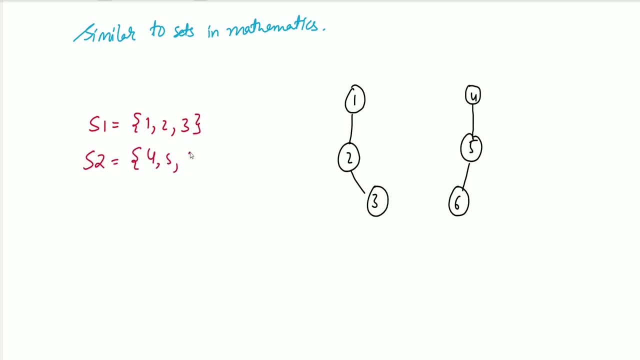 and another set, S2, which will contain my another set of vertices 4, 5 and 6.. Now this is called disjoint, because if you do S1 intersection S2, you will get 5.. So all the disjoint sets, if you do intersection between any two or all of them, you will get 5.. And basically there are two operations. 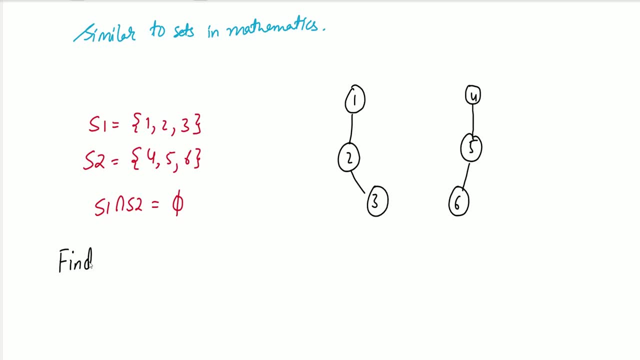 that happens on them. One is find operation. It tells the set to which an element belongs. So it is basically if it is a part of which set. So if I do find 1 in this, then 1 will give. 1 is here, so 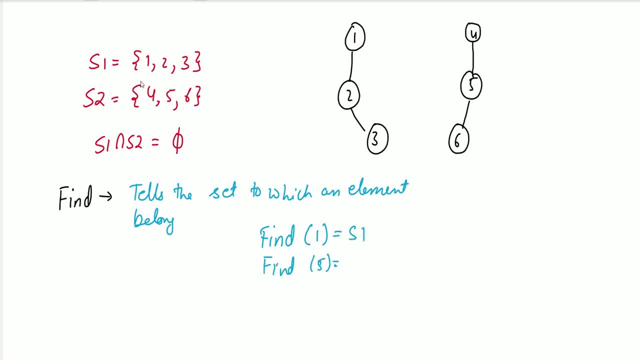 it will give S1.. If I do find 5, so 5 is 5 is not in this set. 5 is here, so it will give you S2.. And similarly, you can run this on different elements and you will get to which set they are belonging. 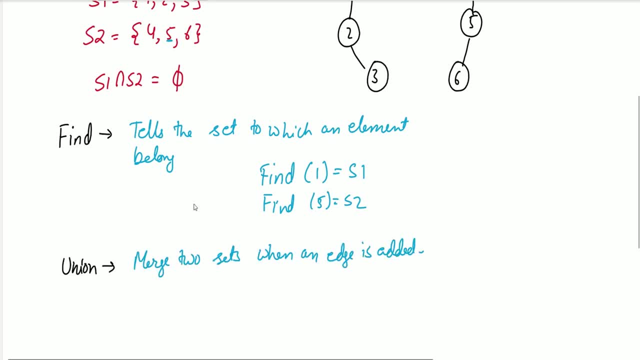 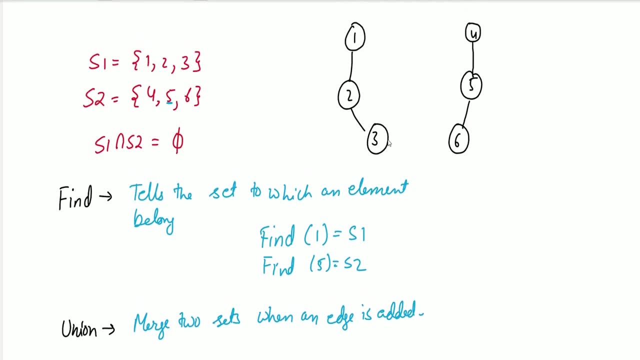 Another operation that it supports is union. So basically it merges two sets when an edge is added. Right now these two are disjoint sets. Suppose I add an edge from 3 to 5. So I'll do first find 3.. Find 3 is S1. Find 5 is S2. So both of them belong to different sets. So we can perform union. We. 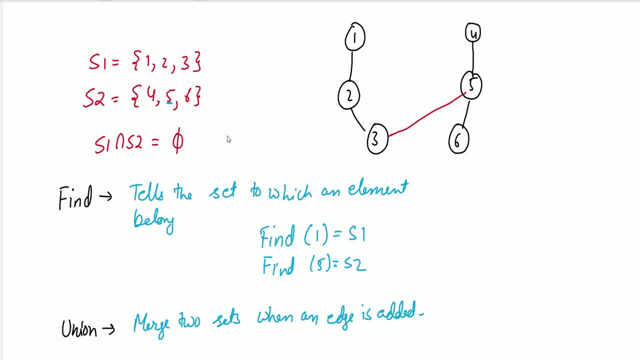 cannot perform union when they both belong to the same set. So when we perform union, union is S1. So here we will do S1, union, S2, and this will give me another set, S3, which will have 1, 2, 3, 4, 5, 6.. 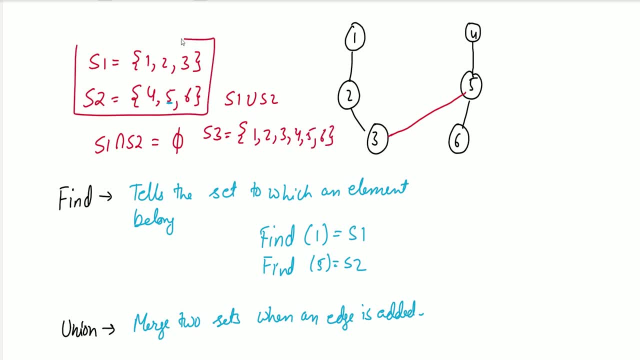 Now, since we have performed union, now we will not have this set. This set vanishes and only S3 will be there, Right? So this merge operation merge two sets when there is an edge, that is, when an edge is added between them. Now suppose I try to add an edge from 1 to 4.. So there will be a cycle created. 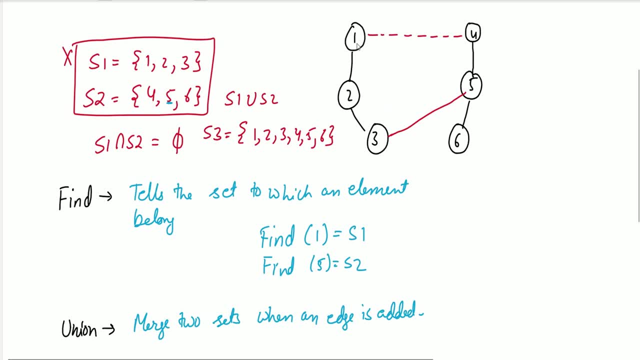 This disjoint set detects a cycle. So now, first we will do find 1.. Find 1 is where in S3.. Now we will do find 4.. Find 4 is there here in S3. Both belong to the same set. If both belong to the same set. 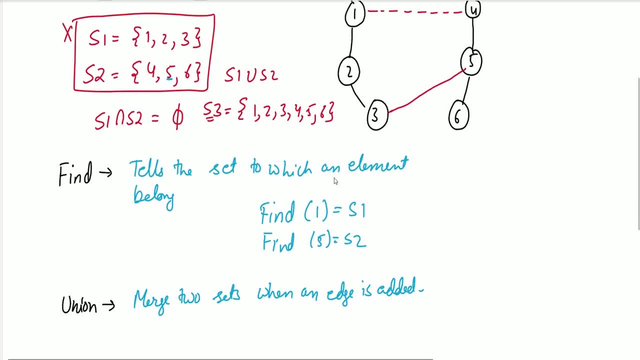 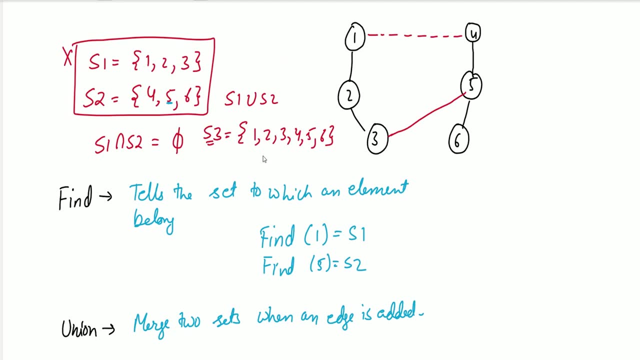 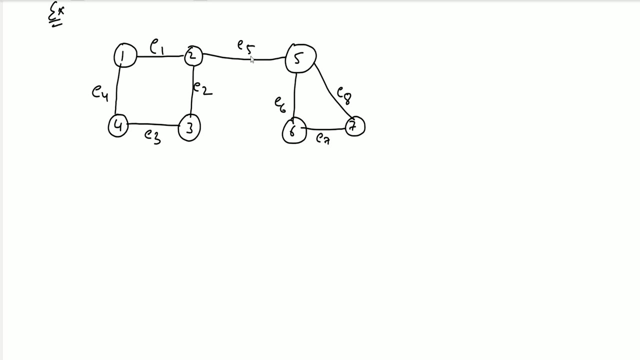 then adding an edge will create a cycle. Here. this is how it detects a cycle. So when both the elements belong to the same set, then adding an edge will create a cycle. Let's take an example to understand this better. Let's take this example in which we have 7 vertices and 8 edges. The vertices are named from 1 to 7, and 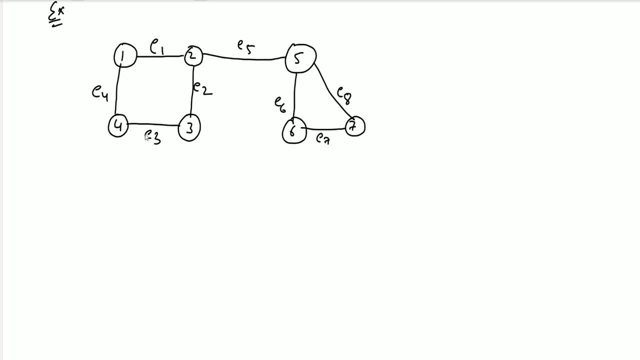 the edges are named from E1 to E8.. So initially what happens is that we have a universal set. In the universal set we have all the vertices and it happens such that we can take any two vertices from the universal set and we can merge them and create a set. So now we will add edges one by one. Let's: 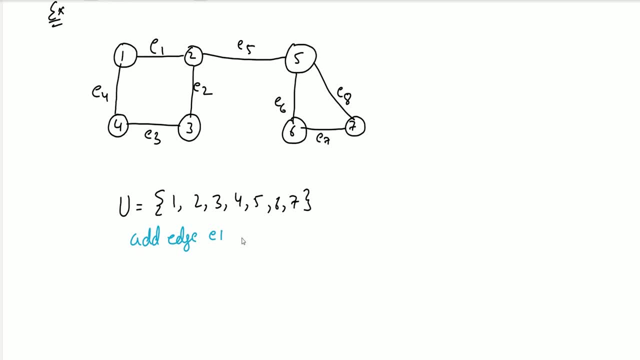 go again sustain these 2 vertices. So here we have an edge 1 and after this we have 1.. So first we will add edge E1. We need to know whether we can select this edge or not. So E1 is from U to V is one to 2.. What we will do, We will. 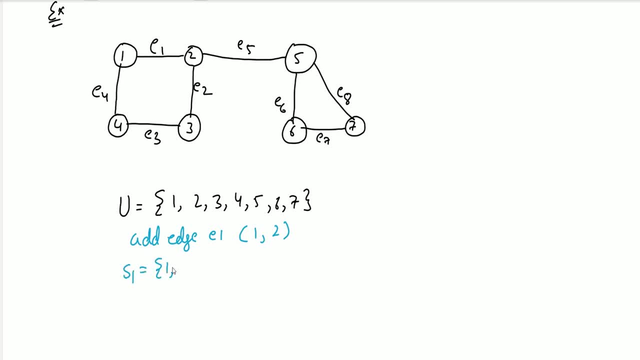 see find 1.. 1 is in universal set. Ok, find 2. 2 is also in universal set, so we can union them and we will create one set, 1 comma 2, and 1 and 2 are not here. 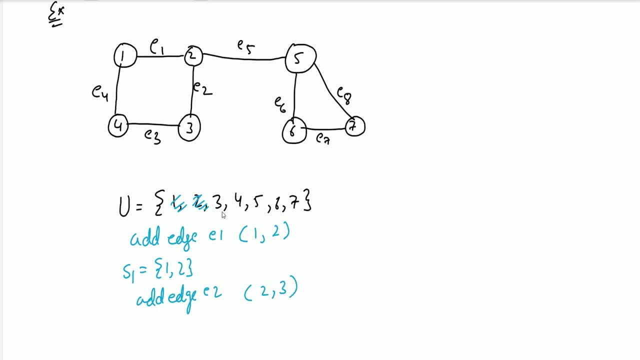 Next we will take edge e2.. E2 is having 2 to 3.. Now we will see 2 belongs to S1.. 3 belongs to universal set. So when we will look at edge e2, it is having two to 3.. Now we will see that two belong to S1,, 3 belongs to universal set. So when we will look at edge e2. next, 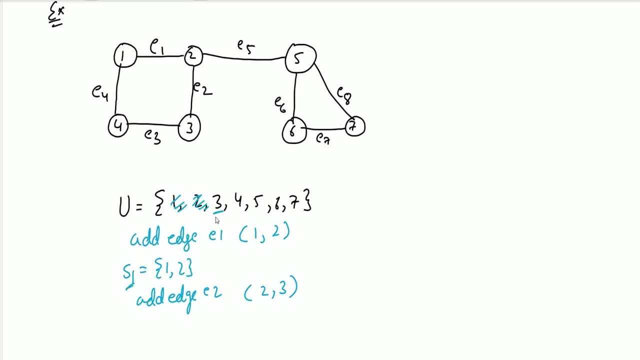 do find two, we will get s1, and when we do find three, we will get universal set so we can add them and we will have s1 union three. so it will give us one, two and three. next, when we add edge e3, we will have three to four. now three belongs to s1, four belongs to now. three will not be here. 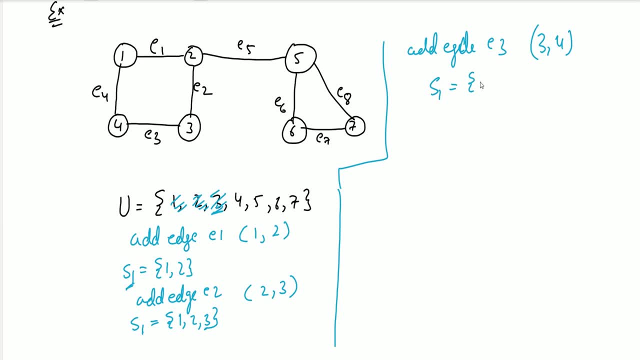 and four belongs to universal. still we can union them and we will get one, two, three and four. now, when we try to add edge e4, e4 is one to four. now we'll do: find one, find one will give us s1. find four, find four will give us s1. now, adding edge one and four will create a cycle. so we have selected. 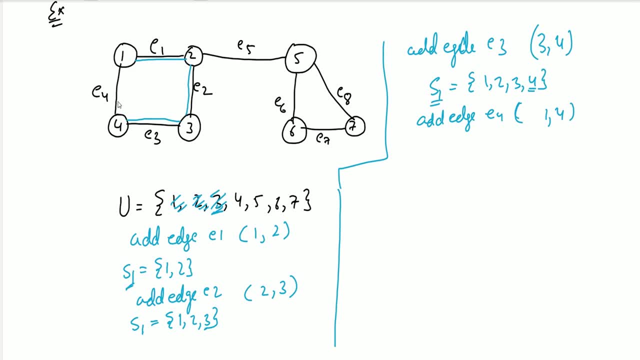 this edge, this edge and this edge. we cannot select this edge. if we can select this edge, it will create a cycle. okay, so here we can say: cycle detected. now we can add edge in any order, that it does not matter. we can add first e8 also. so let's add edge e8. e8 is five to seven, so five belongs to universal and 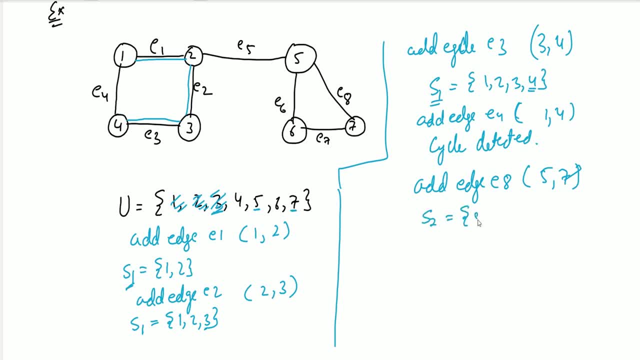 seven also belongs to universal, so we can create another set with five comma seven. now we can add e6. e6 is five comma six, so now five. now this five and seven will not be here. five belongs to s2, six belongs to universal, so we can just apply union on them and we will get five, six and seven. 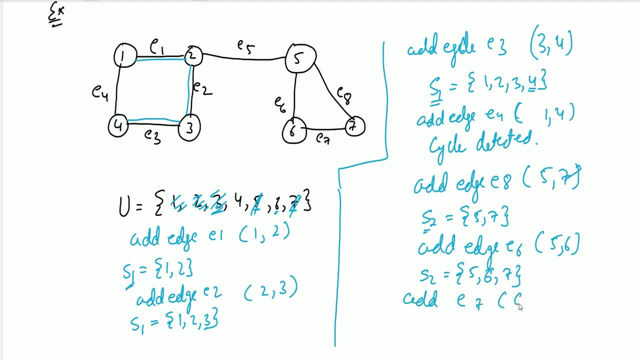 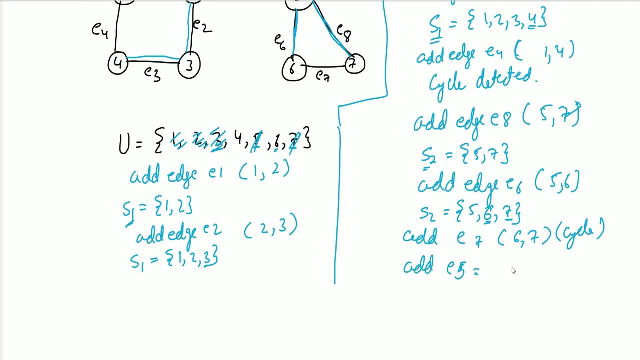 now, when we try to add e7, which is from six to seven. now six belongs to s2, seven belongs to s2. so now adding this will create a cycle. and you can see that if i add this and this, e6 and e8, then adding e7 will create a cycle. so we can say cycle. now last edge remains if we add e5. e5 is from two. 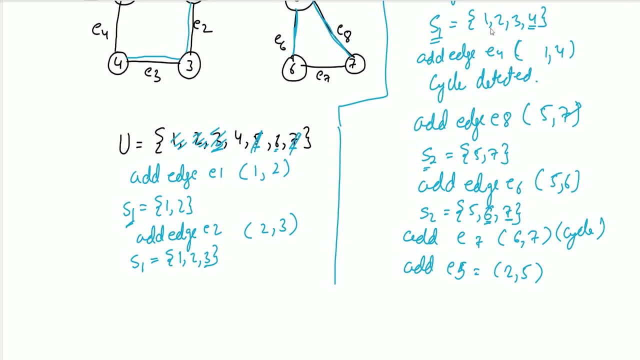 5.. So 2, if we do find 2, we have S1, because 2 belongs to S1 and 5 belongs to S2.. So now they belong to different set, So we can apply union on them and we will get 1,, 2,, 3,, 4,, 5,, 6,, 7.. So here: 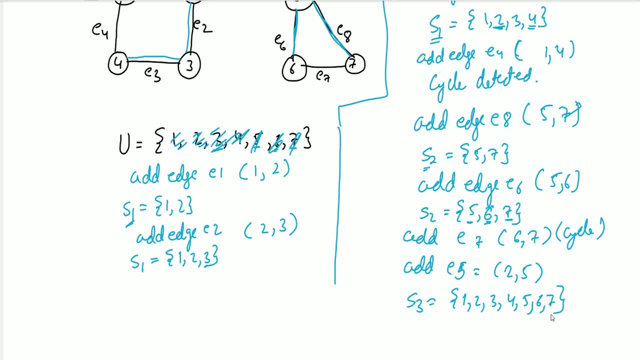 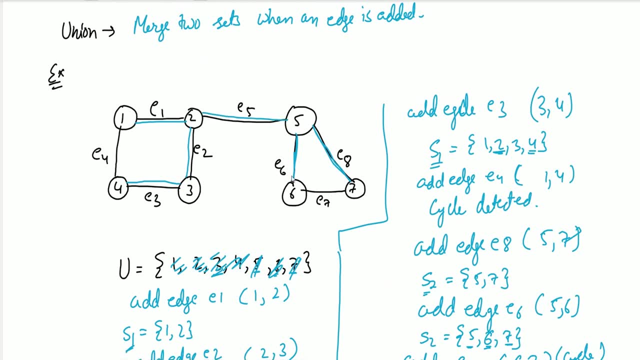 in the universal set. there is nothing left and all of our vertices are in S3. So we have selected this also. Now you can see that there will not be any cycle if we have selected this And if we try to add even one edge, even if I try to add a new edge from 3 to 5, 3 to 6,, 4 to 7, any edge in this. 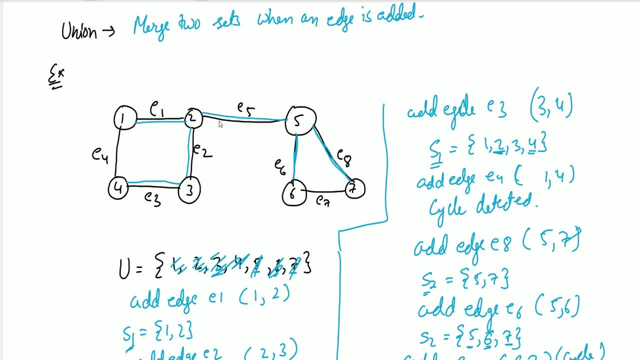 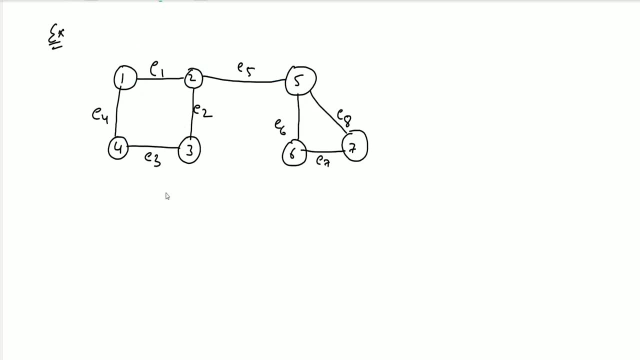 will create a cycle. This is the minimally connected graph here. Now let's see graphically how this will happen. Now let's see how this can be done graphically. So initially let's see we do not have anything. Let's say, we try to add edge. even What will happen? We will have 1 here. 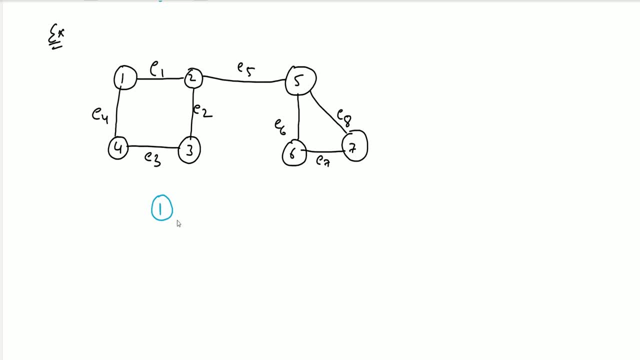 and right now what we did was we were naming the set. But in algorithms we do not need to name the set, We just need one representative element that can represent the whole set. So what will happen when we try to add edge? even we will have 1 and 2, and 2's parent will be 1.. So this is how graphically it will work. 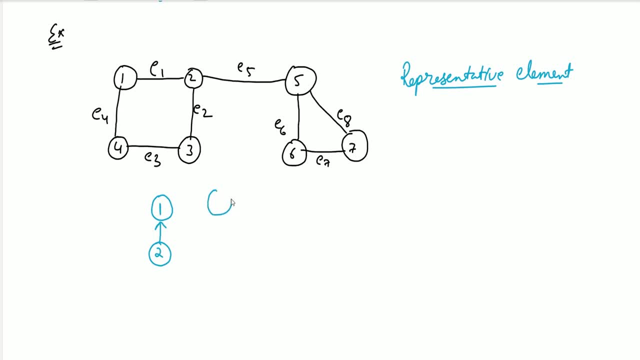 Now let's suppose we try to add E3. So now we will have 3 and its child will be 4.. And next, let's suppose we try to add E3. So now we will have 3 and its child will be 4.. And next let's suppose 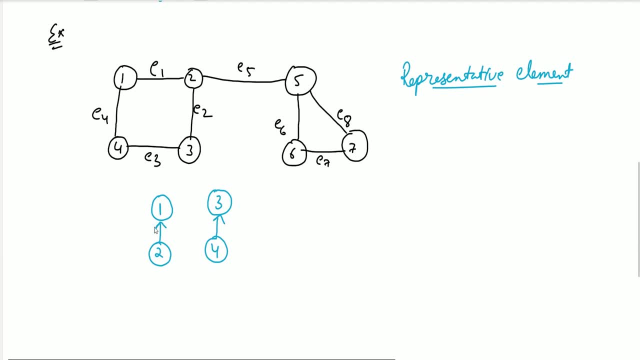 we try to add 3 and its child will be 4.. And next we will try to add 2 and its child will be 5.. And we will see how the sets are detected Now. now we will see: 2's parent is 1.. 1 does not have any. 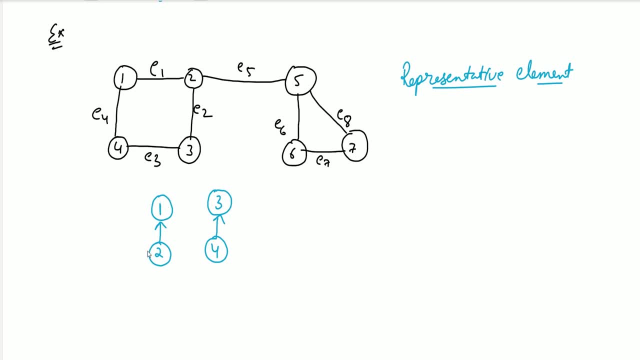 of 5 is alone right now, So it means they both belong to different set. why? because the representative element of 2 is 1 and the representative element of 5 is right now 5, itself. So now what we will do: we will add the parent of 5 as well. Now you can ask why the parent of 5 as 1. Because now we know that of 5 is 1.. So we know this number. So now we can guess what the power of the 3 gives per 1.. Because mày, by analysing what the value, and that was 1 plus 1 plus 1 plus 2 plus 1 plus- 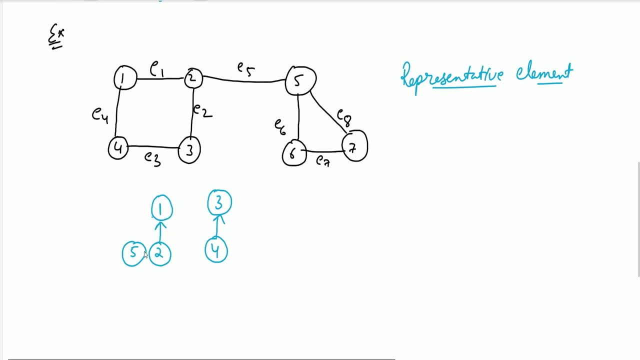 Because when it was not there, there were two elements in this set and there was only one element in 5. So what we do is we do union by rank or union by weight. So when we have more element in one set, then the another set's representative element will change. 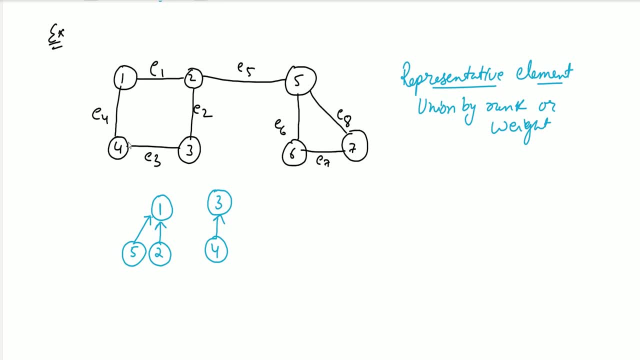 So the representative element of 5 will become now 1.. Let's suppose we try to add 1 and 4.. So what is the representative element of 1? 1 itself? what is the representative element of 4? 4's parent is 3.. 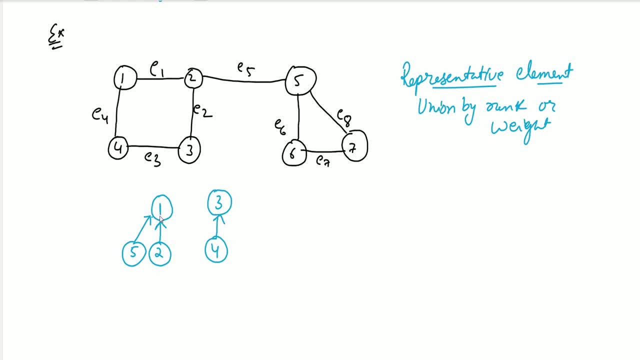 So 3 is the representative element of this and 1 is the representative element of this set. So 1 and 3 are different. So it means we can add E4 right now. And what will happen? We can just set the parent of 3 as 1.. 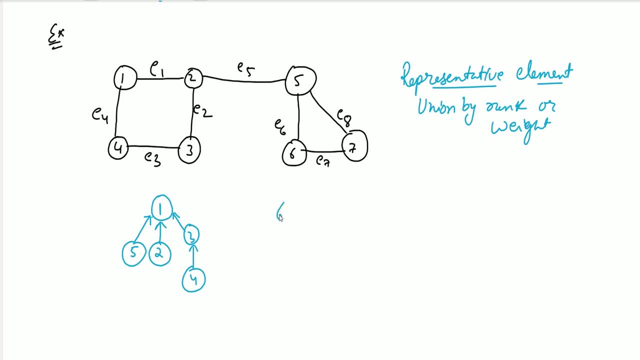 Next, let's suppose we try to add E7. So this will become 6 and 6 parent will become 7.. Now we try to add E8. When we try to add E8, E8 is between 5 and 7.. 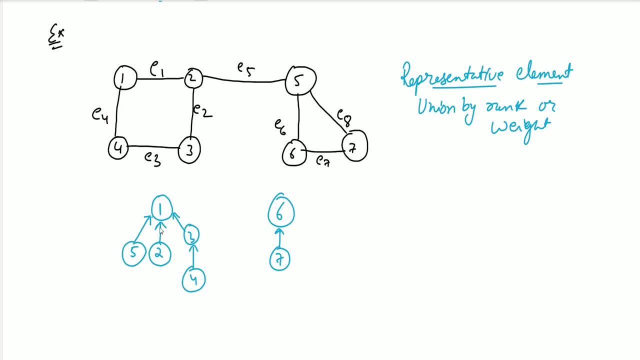 So 5, 5's parent is 1, 1 is the representative element of this set. 7, 7 parent is 6, so 6 is the representative element of this set. So now, when we add this and we do union by weight, we add it like this: 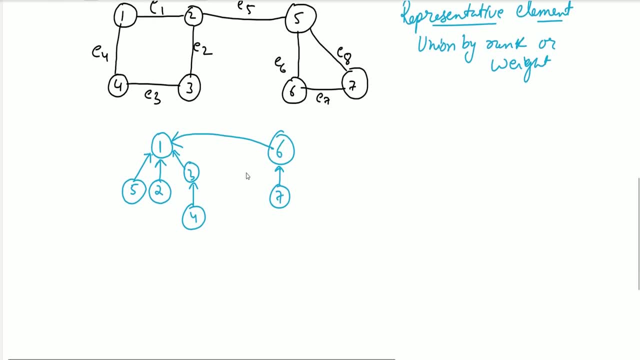 And this is how graphically it works: To find. what find will do? Find will go to the root and it will find the parent And union. what union will do? Union will see which area Which is greater in rank and will make another the child of the one which is greater in rank. 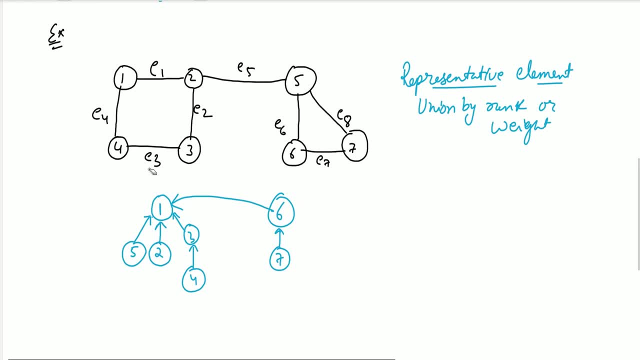 Now this may seem difficult, but it is very easy when we use array. Let's suppose this is the array and each element represents a vertex here, So we can, and the name of this array is parent. Basically it is telling who is the parent of which vertex. 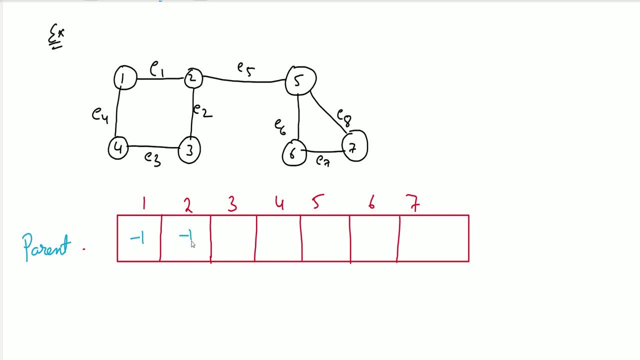 So here, initially, what we will do: we will put minus 1 everywhere. Why minus 1?? Because what I'm going to do is I'm going to define the weight by this negative number. So if something is minus n, it means that there are n vertices in that tree. 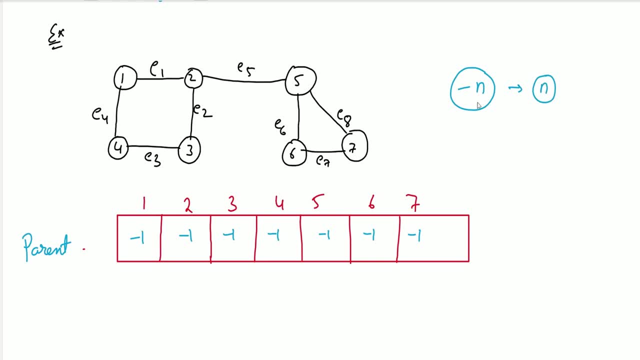 And what will happen when we get the negative number? It means that number is the root. So right now, every number is the representative element of itself or it is the root of that tree. Now let's try to add 1 and 2. when we try to add 1 and 2.. 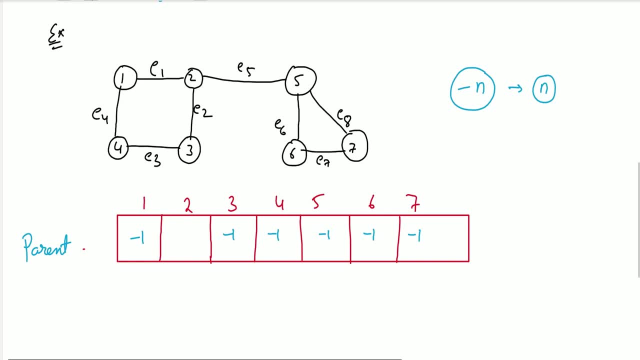 So now what will happen? The representative element of 2 will become 1, and here we will do minus 2.. OK, so we will do just union and we will do minus k. Now let's see, Let's say we are trying to add the edge E3, which is between 3 and 4.. 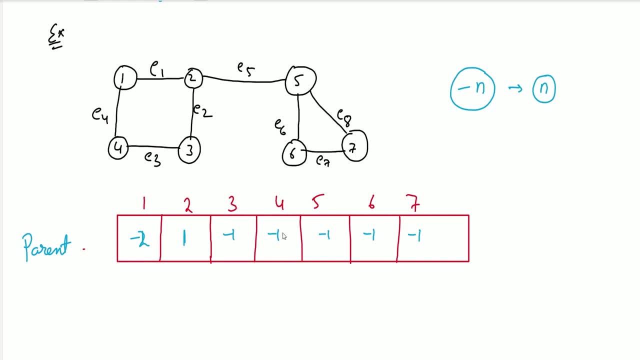 Parent of 3 is minus 1 and parent of 4 is minus 1.. So what we will do? we will just change the parent of 4 to 3 and we will make this minus 2.. Let's suppose we try to add 2.. 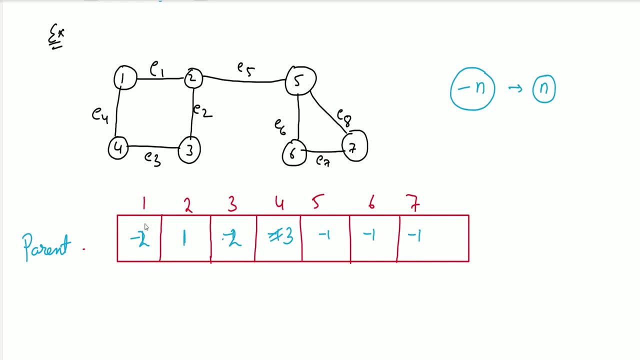 3. Now, parent of 2 is 1,. parent of 1 is minus 2.. We get minus 2.. It means 1 is the representative element of 2.. Parent of 3 is minus 2.. We get minus 2.. 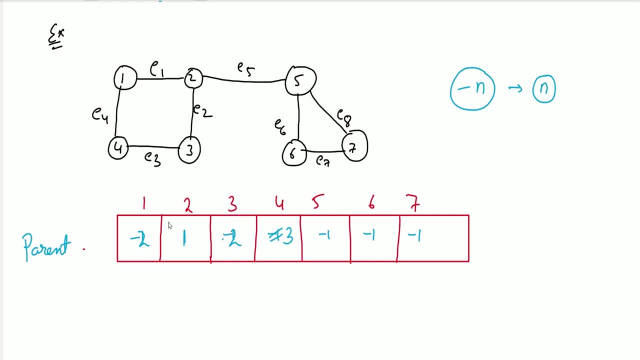 So it means 3 is its own representative. So now we can union them, because both came out to be negative. So what we can do, we can just change this to 1 and we can just add this: minus 2 and minus 2.. 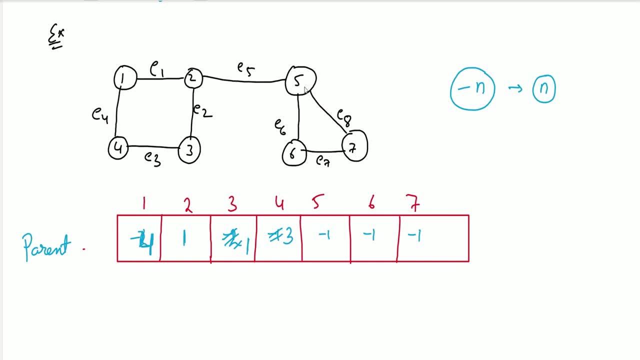 It will become minus 4.. When we try to add the edge between 5 and 7, let's say, parent of 5 is minus 1 and parent of 7 is minus 1. So they both are negative. It means they both belong to different set. 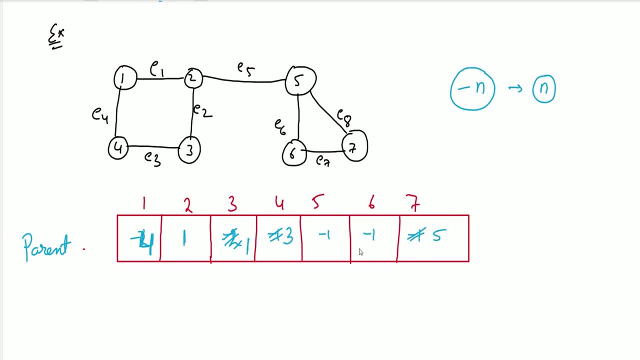 And then we can just do this: We can change the parent of 7 to 5 and we can just add minus 1 to this. This minus 1 will be added here In the previous minus 1, it will become minus 2.. 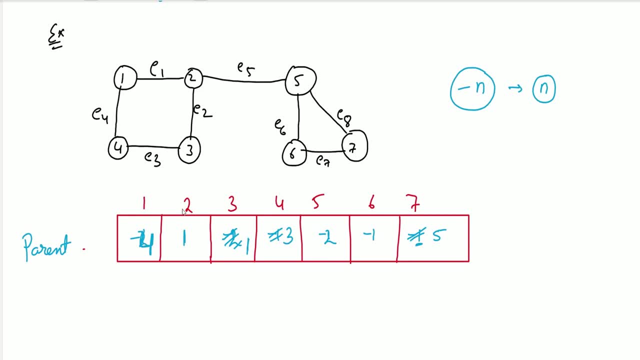 Let's suppose we try to add 2 and 5.. So 2 and 5.. 2's parent is 1.. 1 parent is minus 4.. So 1 is the representative element of this and 5's parent is minus 2.. 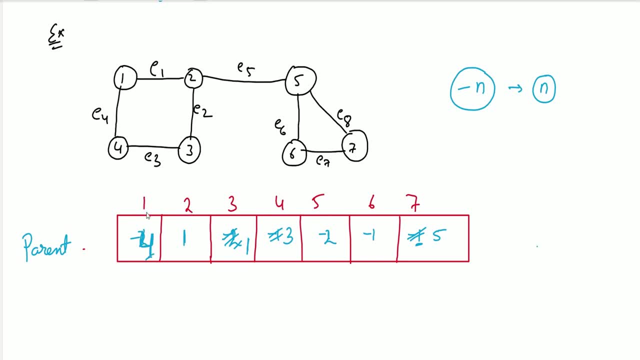 It means 5 is the representative element of this set. We are doing union by weight. So what will happen? We will see the weight of 5, which is minus 2.. The weight of 1, which is minus 4.. 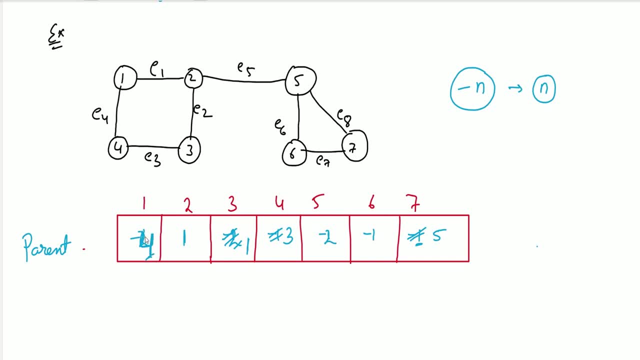 It means the 1 has more weight. Why? Because if we transform this minus 4, then we know that there are 4 vertices in this tree and there are 2 vertices in this tree. The 2 vertices are 5 and 7.. 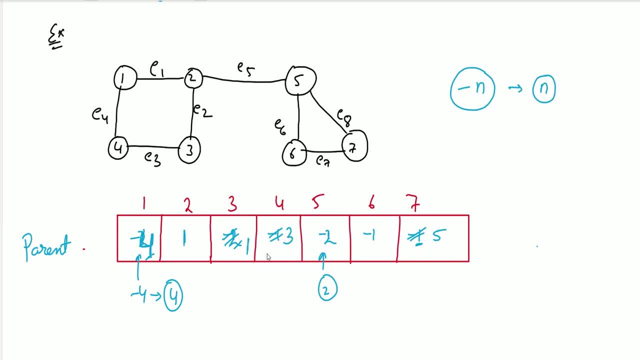 Here the 4 vertices are 1,, 2,, 3, 4.. So when we merge them, what will happen? The parent of 5 will become 1 and this will become minus 6.. Now suppose we want to add the edge 6, 7, which is E7.. 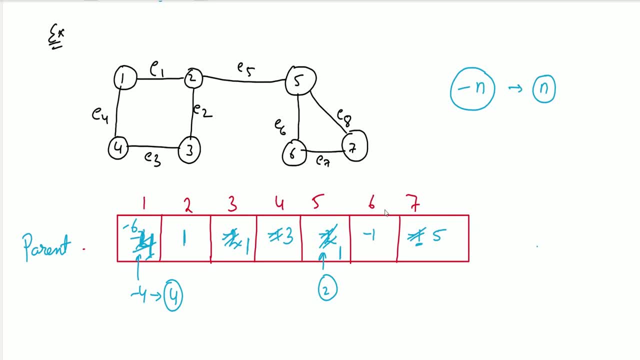 So the parent of 6 is minus 1.. It means 6 is the representative element of this set. The parent of 7 is 5.. The parent of 5 is 1.. The parent of 1 is minus 6.. 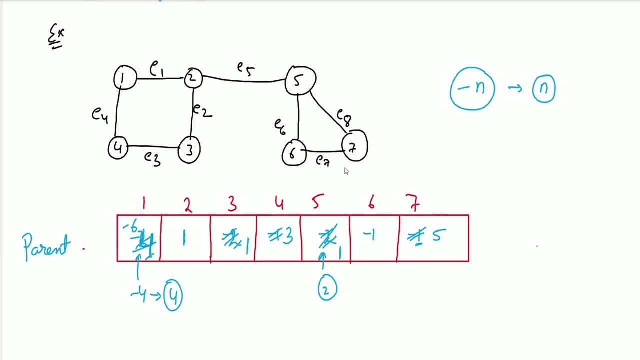 It means 1 is the representative element of this set. Both the sets are different, So we can just add the parent of 6 as 1 and we can just do minus 7.. Now all of them belong to the same set, right. 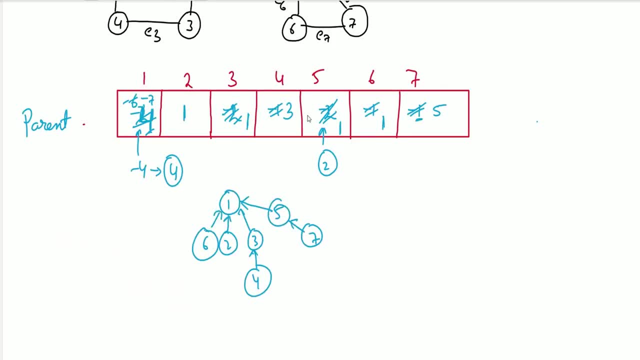 And we can draw them also like this. And if we see this array, then we can see that we are getting this representative element of the set in almost constant time. And this gives us a very beautiful solution because it will take either 1 or 2 steps only, right. 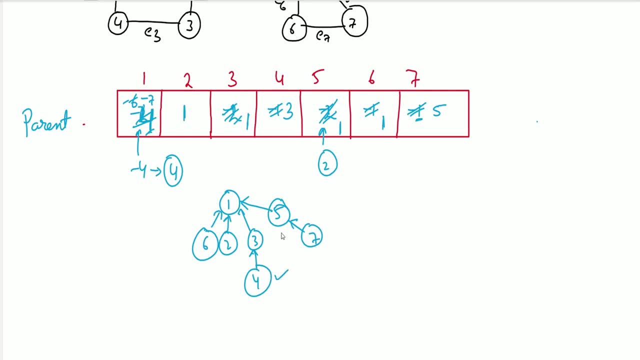 Sometimes it happens like this: 4. This is taking more steps than other. This 7 is also taking more steps. So what we do is we use collapsing find. What happens? Suppose I call find on 7. So 7's parent is 5,, 5's parent is 1, 1's parent is minus 7.. 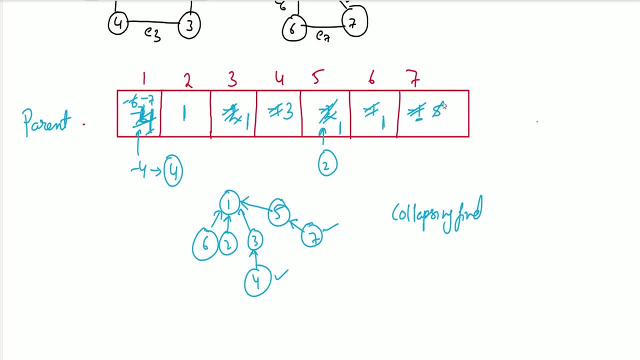 It means 1 is the representative element of this 7.. So what we do? we just change this 5 to 1.. So here what will happen? We know that 1 is the representative element of 7. So we just do this. So, while doing, find we can do this. 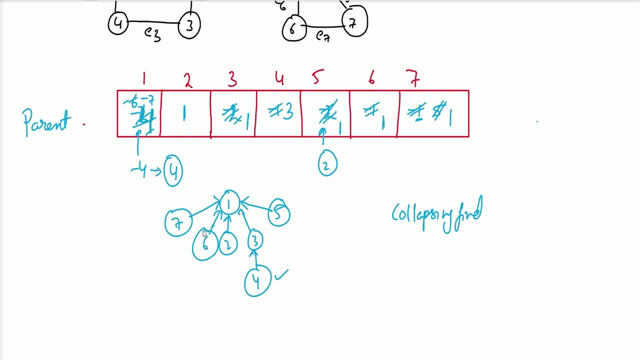 So first time it may take more steps, but next time it will take less steps. And similarly, if I do find 4,, 4's parent is 3, 3's parent is 1, 1's parent is minus 7.. 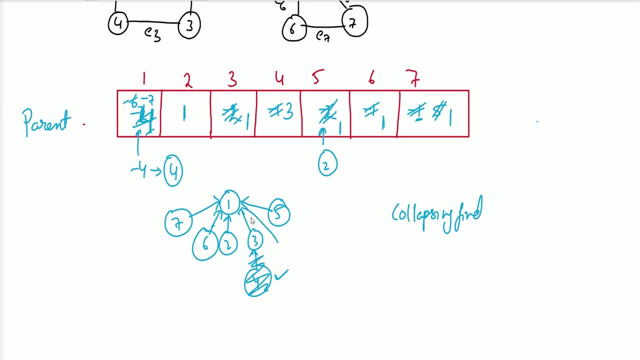 1 is the representative element. So we can remove 4 from here and we can directly put it here. So this is called collapsing find. So it reduces the time when we search for the next time. First time we are searching for anyone's parent or we are doing finding. 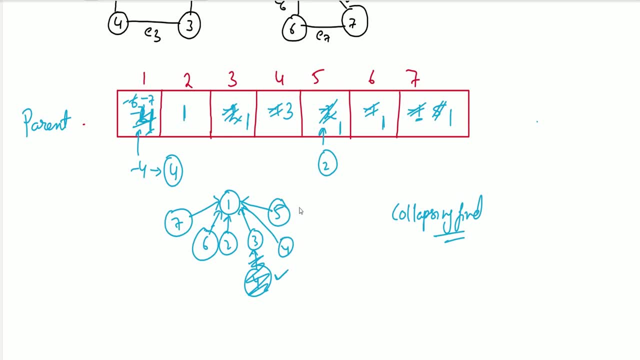 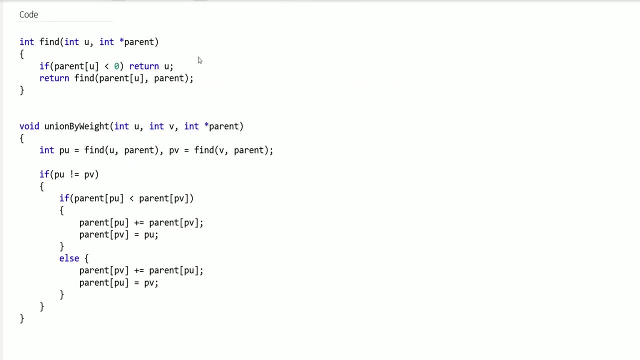 it will take the number of steps that it usually takes, But next time it reduces that time. OK, let's see the code. So the code of find and union by weight is very simple. They are just few lines. So here, what I did is I made a parent matrix containing the elements. 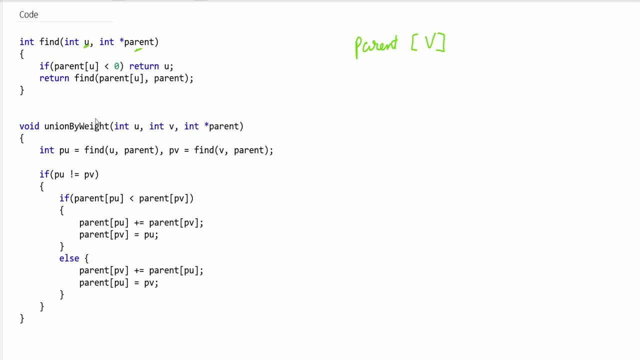 And in the find I'm passing that. So it is you and parent. So if parent of u is negative, as we see there, so we have to return u. It means u is the representative, And if parent of u is not negative, then we need to go further and we need to check it. 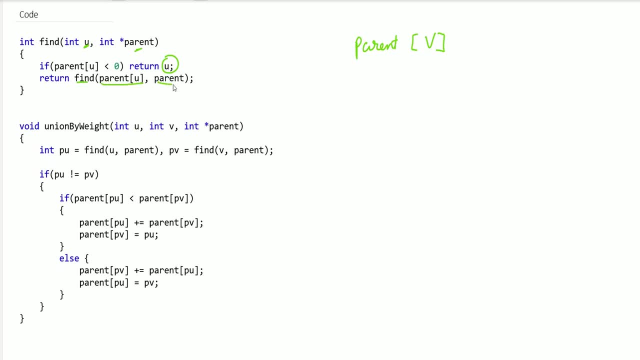 So we will just call find with parent of u and parent matrix will be passed as it is. So what we are doing? suppose there are three nodes: one, two, three, Its parent is minus five or minus three, Its parent is one, its parent is two. 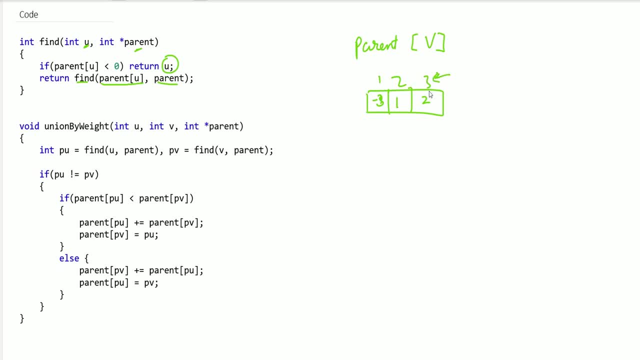 So we want to call find on three. So we call find on three. The parent of three is not negative, So we'll come here and it will call find. parent of u means parent of three is two And parent matrix will be passed as it is. 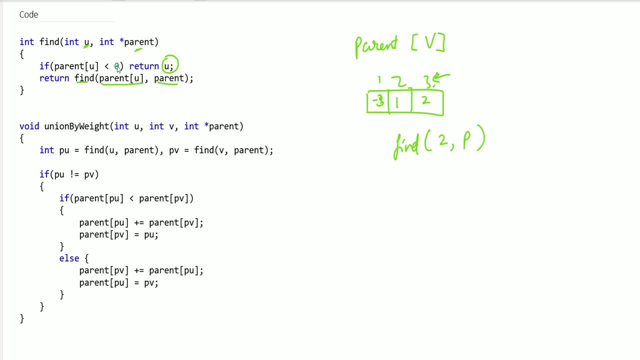 Then we will go here: Parent of two is one, which is not negative. So we will call find again with parent of two. So find parent of two is one, and parent matrix will be passed as it is. Then we'll call parent of one is minus three, which is negative. 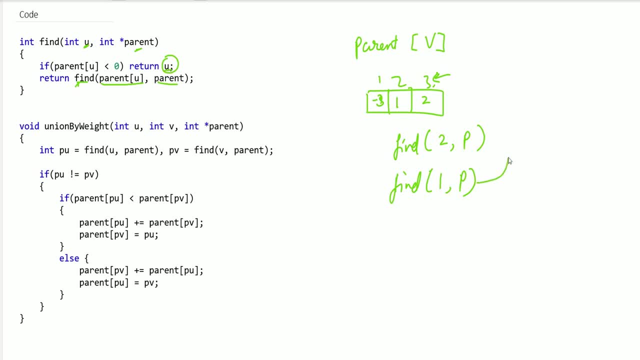 So parent of u is negative, So we will return one. So this will return one here And this because of this return, it will return one to the calling function. So find three comma. parent will return as one And we can see that one is the root node of this set or is the representative element of this. 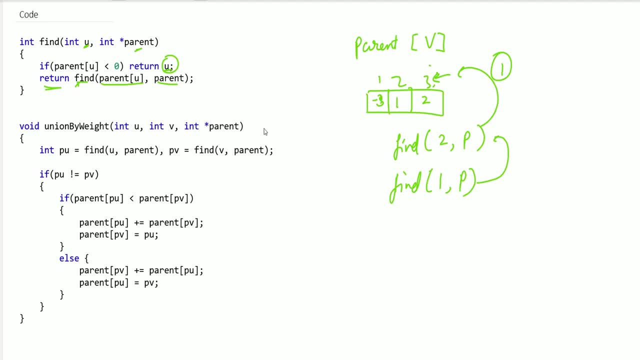 And we can see that one is the representative element of this set. Now next is union by weight. So union by weight. we pass two vertices, u comma v, on whose set we want to apply union and a parent matrix. So first we will. 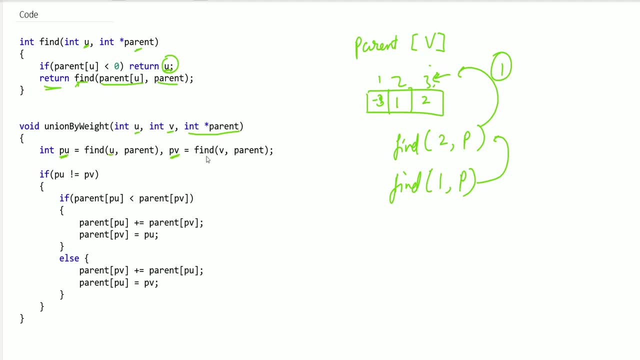 Find the representative element of u and representative element of v And if both of them are not equal. So we perform union only when the parents are not equal. But we cannot let it in the user's hand that they will check whether the parents are equal or not. 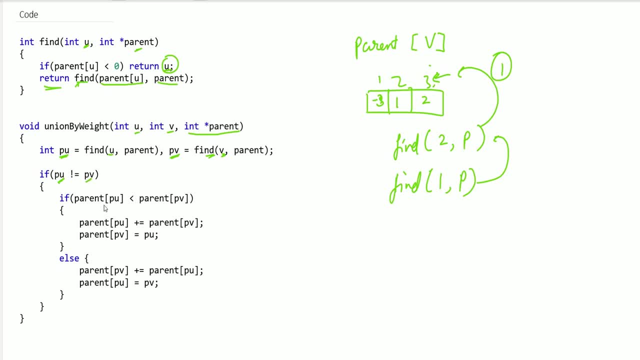 So here we will check that if the representative elements are not equal, then we will check if parent of p? u is less than parent of p? v. What it is doing is so parent of p? u is negative because p? u is a representative element. 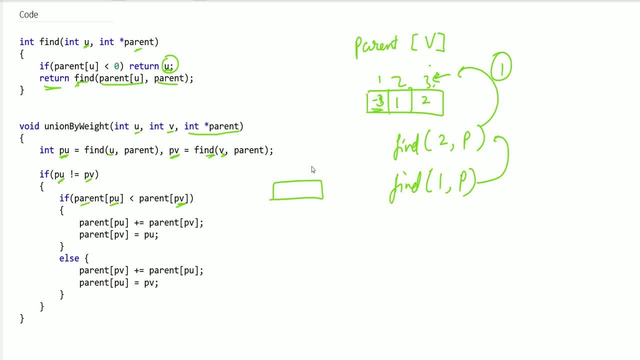 So every representative element in the parent matrix they have negative number. So we are checking if parent of p? u. suppose p? u is minus three and p? v is minus two, It means there are three elements here and two here. So by weight p u is greater than p v. 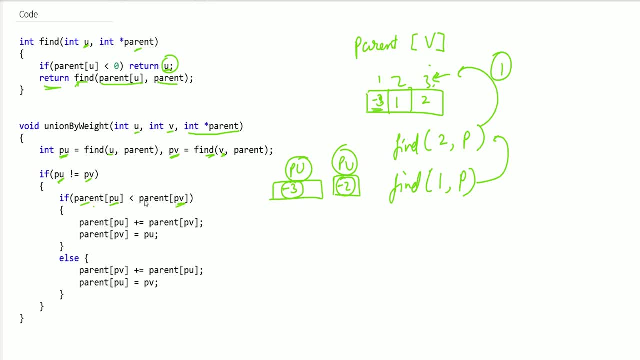 So that is what we are checking. If parent of p? u is less than parent of p v, it means p? u is greater than p v in terms of weight. So what we will do, We will add the weight of p? v to p? u.